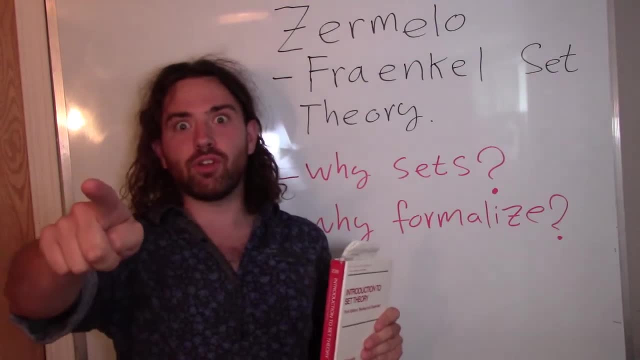 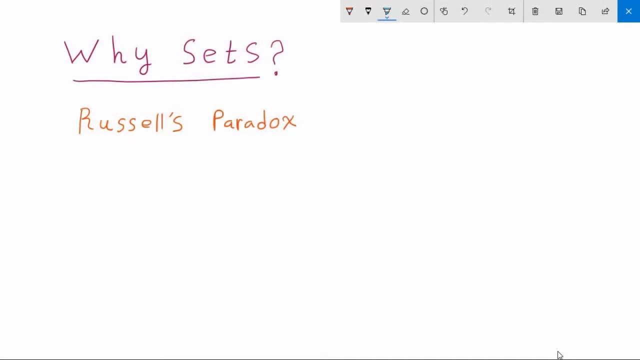 for those of you who want the introduction, it's time to travel to the platonic realm. The first thing I want to discuss in regards to why study set theory or why we need a formal set of axioms involves what's called Russell's Paradox. 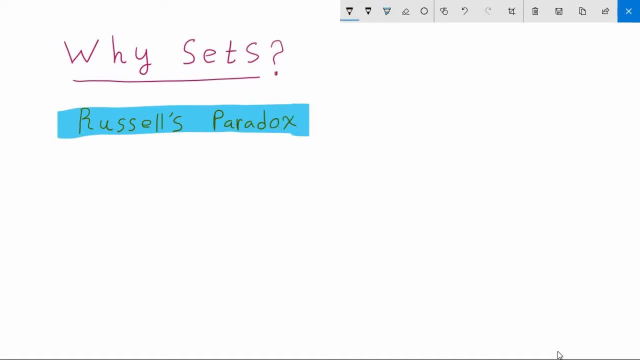 You may have heard of this before, but we're going to review it. So Russell's Paradox shows the pitfalls of what can happen if we just work with a naive set theory that isn't bound by any sort of constraints of an official axiomatic system. So the paradox goes like this: We define: 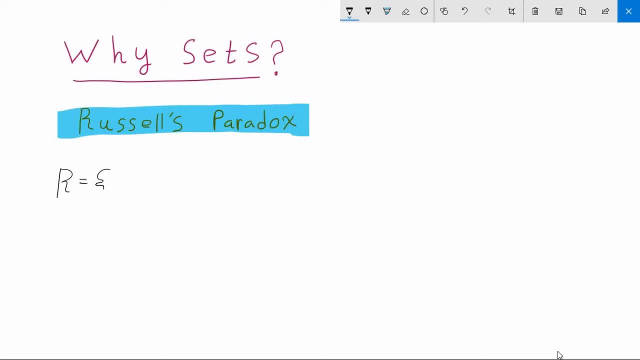 a set R, and this set is going to be the set which contains all other sets, x, such that x does not belong to itself. Now this seems like a pretty reasonable thing to think about. So we know that we can have sets that contain other sets. For instance, I could make: 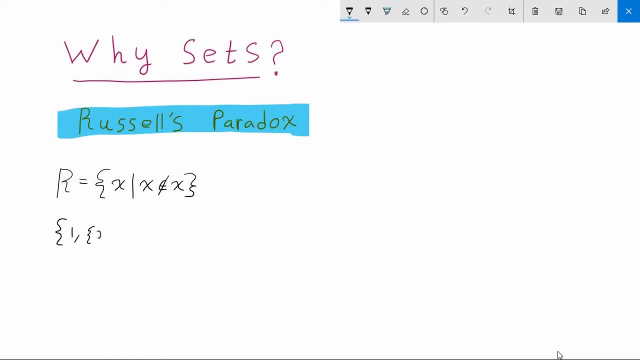 the set which contains 1, and let's say it contains the set 2 and a square. Right. so a set is just some fraction, some sort of bag of stuff from the perspective of naive set theory, and so it can include even other sets, right? So the fact that R is a set which itself contains sets, nothing wrong. 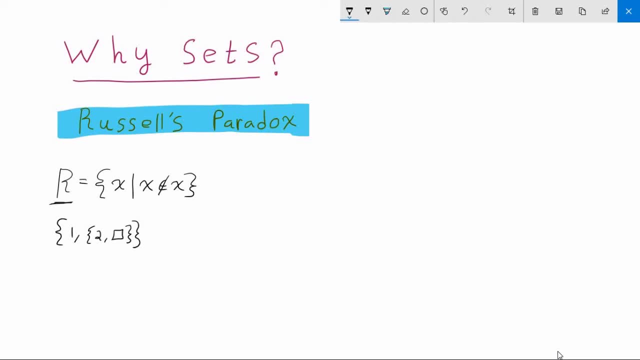 there And the demand that the sets belonging to R do not contain themselves. that's also very reasonable. It's pretty hard to come up with an example of a set that contains itself, For instance, if I wanted to make a set that just contained 1, and I wanted to try and make a set that contained. 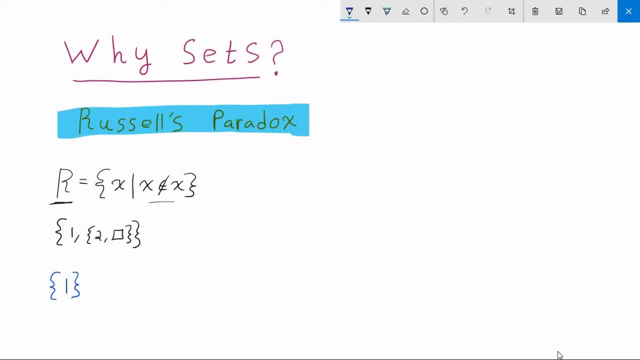 itself. well, I could try and put this set 1, the set containing 1, inside of itself, So I would still have the set containing 1, and inside of that would be the set containing 1.. But now this set doesn't the set referring to that which is the outer curly braces. this set doesn't actually. 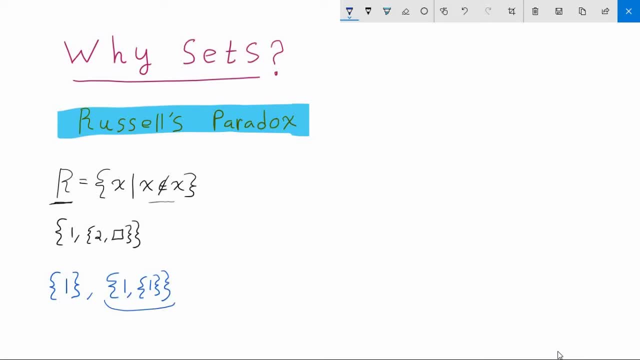 belong to itself, because this is now the set which contains the set 2.. So I could try and put this set which contains both 1 and the set containing 1, and what's actually inside this set is just the set containing 1 and 1 itself. Now this may give you an idea to try and make some set where you had say: 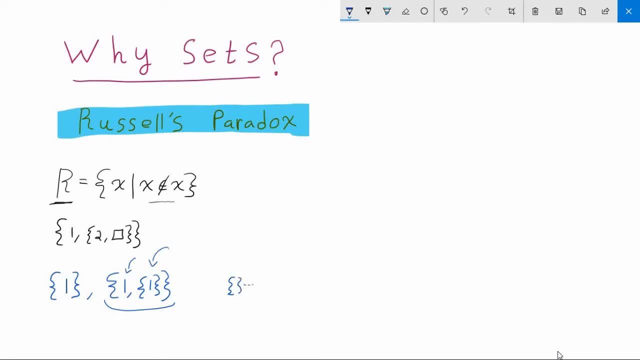 the empty set and then dot dot dot, just infinite nested braces on either side, creating some set with infinite braces both ways. And, okay, this looks like it could be a set which contains itself, but this is pretty unnatural And, in any case, the point is that having this condition, 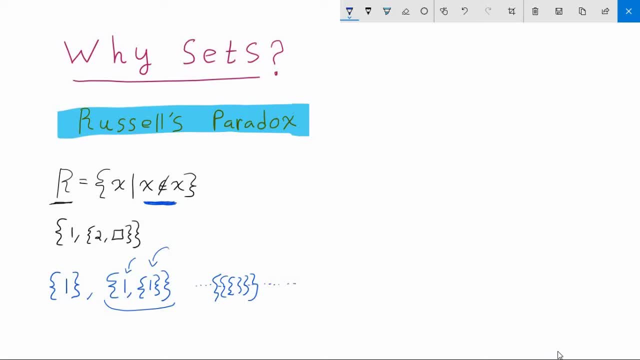 asking that a set not contain itself seems pretty normal. This is basically saying, let's just group all the normal sets together. Those are typically the ones we want to talk about anyways. The issue pops up when we try and ask ourselves a question, and that is: 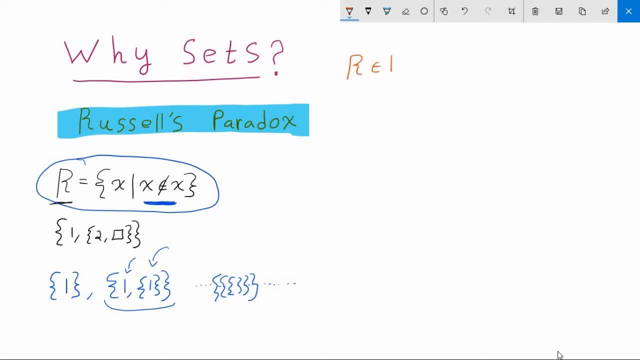 does the set R contain itself. So here's how the argument goes. If this was true, if it was the case that R was contained in itself, that means that it has to obey the rule that it does not contain itself, And so it must be the case that, in fact, R does not contain itself. 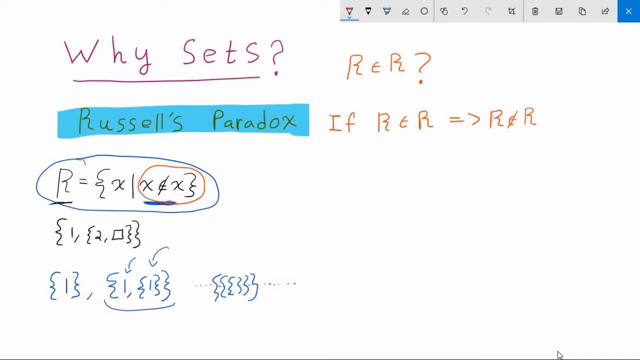 So this seems like a paradox right here already, but this isn't actually a big deal. It would be contradictory for R to both contain itself and not contain itself, but we've just shown that this sort of contradiction only arises if we first assume that it does contain itself. Okay, so no. 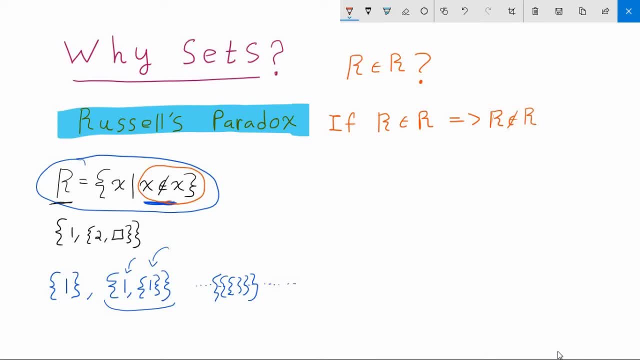 big whoop. that seems ridiculous. So it's got to be the case, then, that R does not contain itself. right, That's got to be the conclusion that we have to draw. But here's the catch: If R does not contain itself, then that means that it does obey the rule, which. 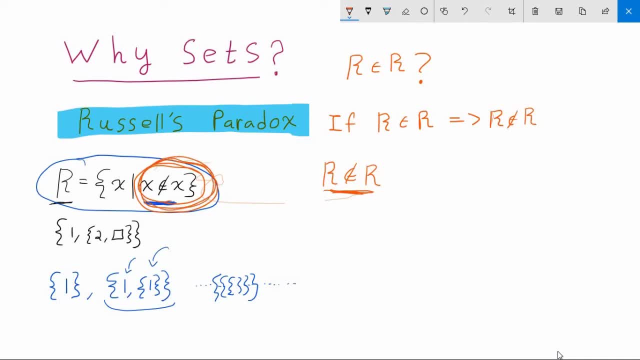 is the defining feature of the set R, And if it obeys the defining feature of the set R, that means, by definition, that R must belong to R. In other words, if R doesn't belong to itself, well then it does belong to itself. Now, if R does not contain itself, then it must be the case that R does not. 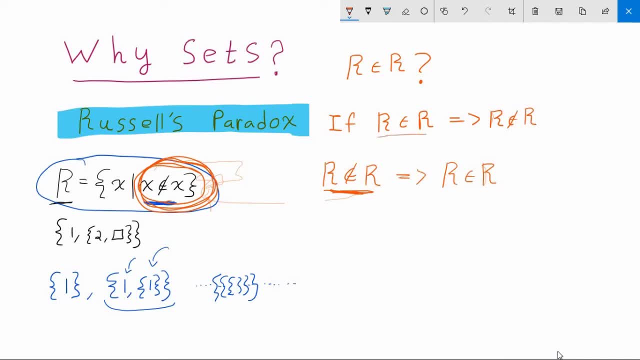 contain itself. Now we've got ourselves a problem because we have that R belongs to itself implies that it does not belong to itself, and if it does not belong to itself, it does belong to itself. In other words, R belongs to itself if, and only if, it does not belong to itself. We now have 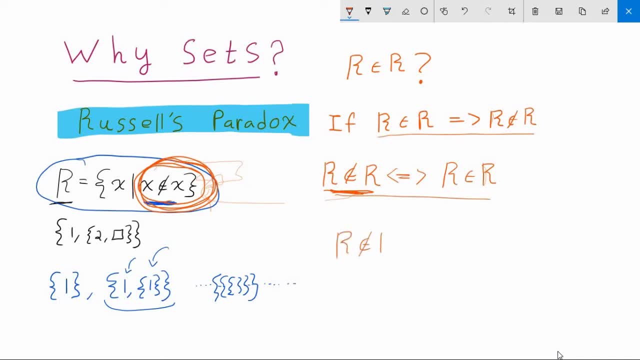 a problem, because this is equivalent to saying that the set R must not contain itself and it must contain itself simultaneously. So this can't possibly be true. First off, this seems frightening for all of mathematics because somehow we've logically derived some sort of contradiction. We've exposed a hole, a paradox in 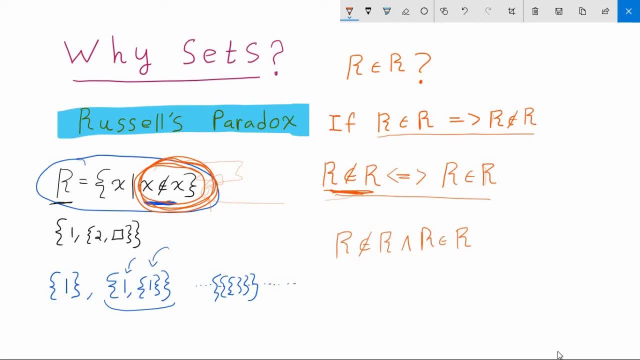 the logic of mathematics itself. And the other fact being is that not only is a contradiction bad enough in itself to have in your theory, well, the very reason why a contradiction is bad is because it follows from any false statement. you can prove any statement whatsoever. Q. 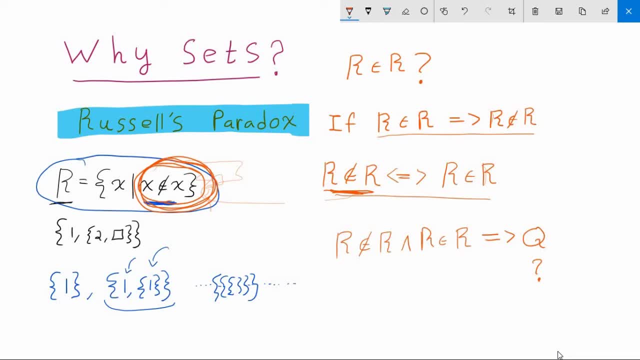 And this is essentially why we don't like contradictions, because from a contradiction you can derive any other statement, and that makes a theory useless. You can prove every single statement true or false, And this is clearly not the sort of logic we want to work with. 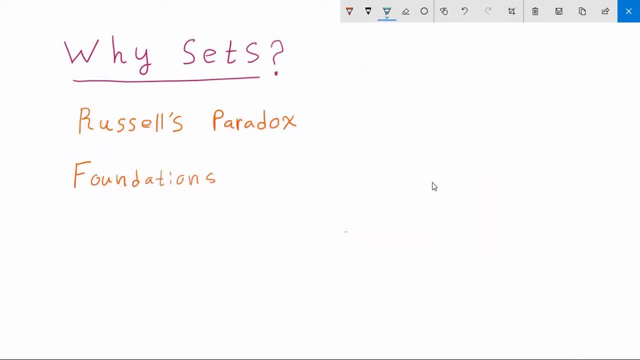 The other reason why we want an axiomatic formulation of set theory is because it's a very complex set theory. The axiomatic formulation of set theory is as a foundation for mathematics. By this I mean a lot of the objects that mathematicians work with, and pretty much at the time of 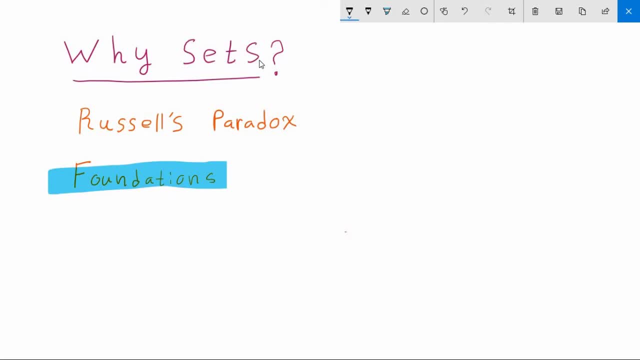 the foundation of axiomatic set theory. all of the objects that mathematicians work with can really be phrased in terms of sets. So the natural numbers form of sets, but even the natural numbers themselves can be described in terms of sets, as can the real numbers, the complex numbers, and so 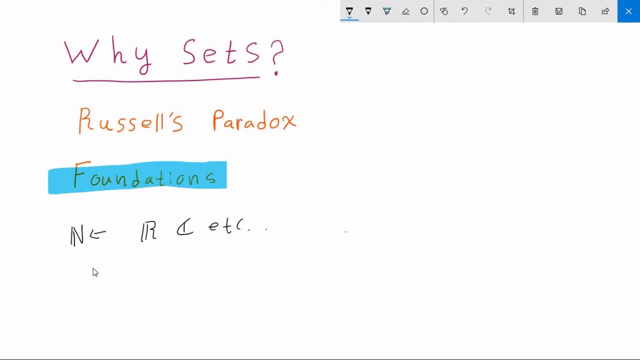 on And lots of times, whether we're studying, say, topology or we're studying group theory, really what we're doing is defining objects in terms of sets and studying functions between them, And one of the things we're going to see in this course is that functions themselves can be described. 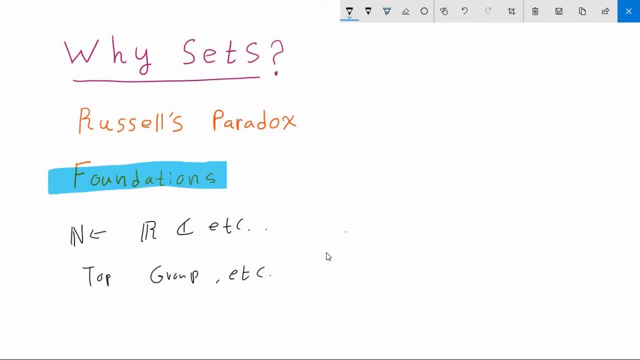 as sets. So we'll sort of notice that a lot of these things can really be put in the framework of set theory. And one of the other things that we do in mathematics is we prove things starting from axioms, which are baseline assumptions. So with any rigorous logical argument, of course, no fact can truly 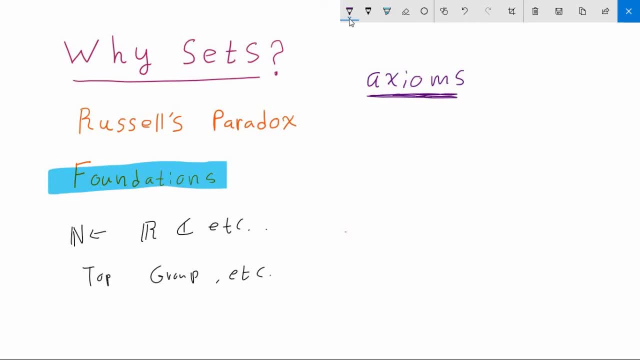 just be derived out of nothing. You have to have some assumption at the bottom of it all. And the idea is: in order for mathematics to have the greatest amount of objectivity, we really want to have a scant collection of axioms. We want to keep it really slim and be able to derive as many mathematical 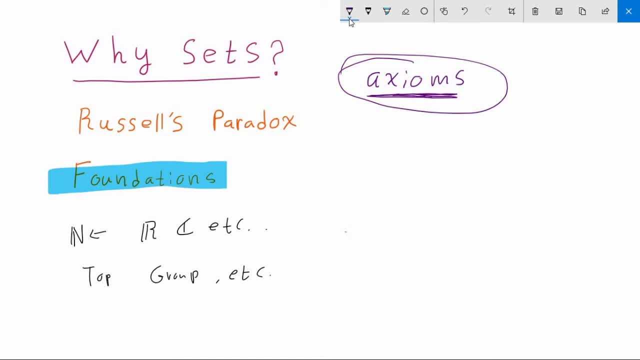